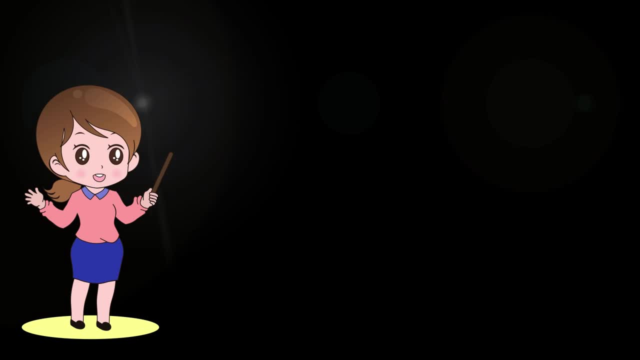 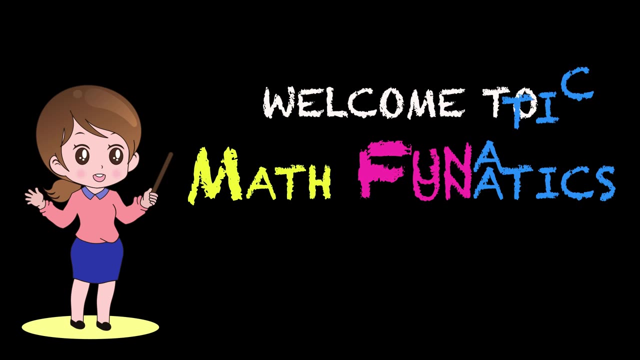 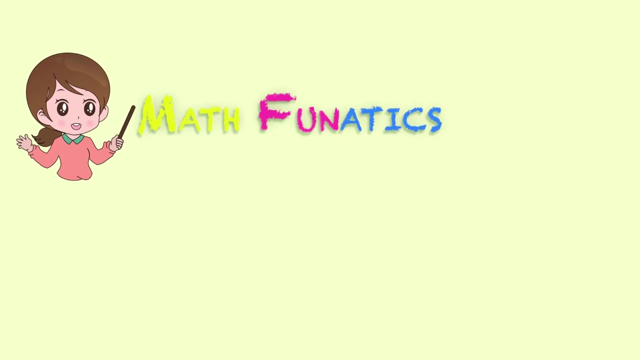 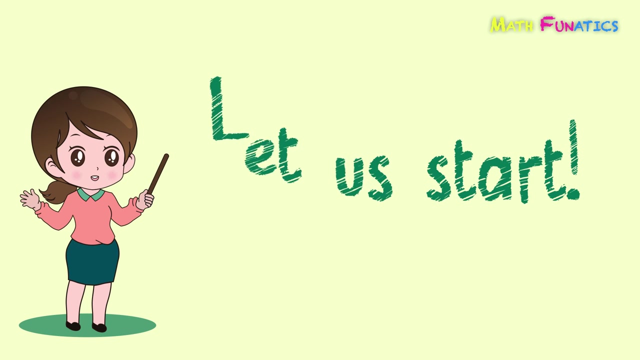 Welcome to MathFanatics. In this video, we'll be learning about integers. To learn what integers are, we need to start with the whole numbers. Let us recall what we basically know about whole numbers. Whole numbers are simply the numbers starting with a zero on the number line. 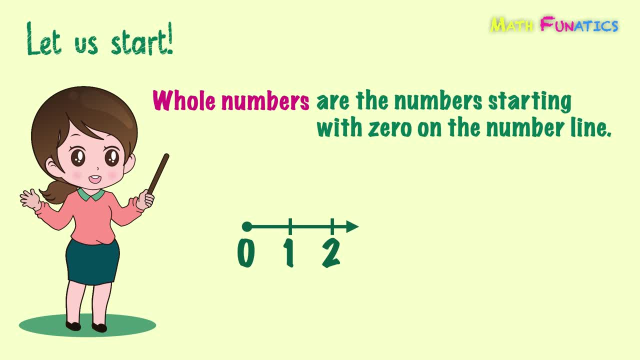 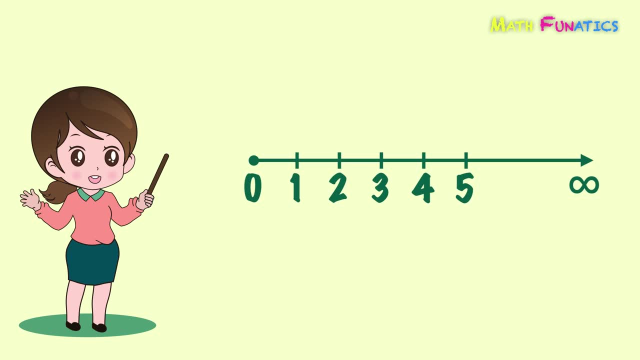 So we have 0,, 1,, 2,, 3,, 4,, 5, and continue all the way to infinity. This number line only shows the numbers specifically on the right of zero, But the truth is the number line actually goes in both directions. 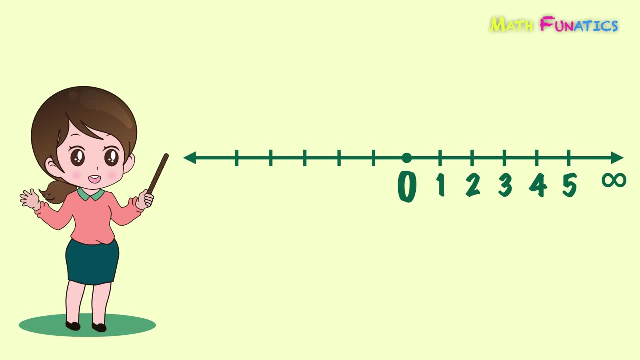 So, aside from the numbers we see on the right of the number line, starting with zero, we also have numbers on the left. These whole numbers on the right, which we knew as the counting numbers, are also referred to as positive numbers On the left of zero, on the number line. are these numbers? 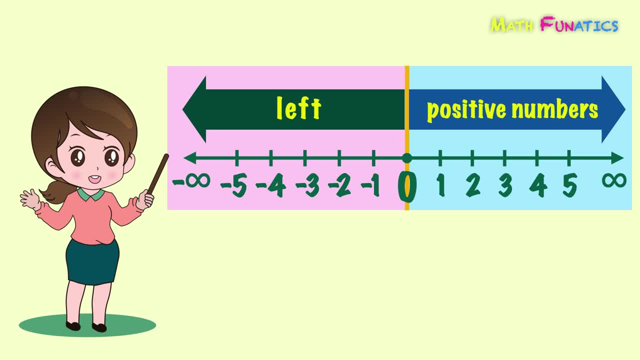 They are just like a mirror image of the numbers on the right. These numbers are referred to as negative numbers. Again, on the right are the positive numbers, while on the left are the negative numbers. Zero, which is found in the middle, is the one that separates the two sets of numbers. 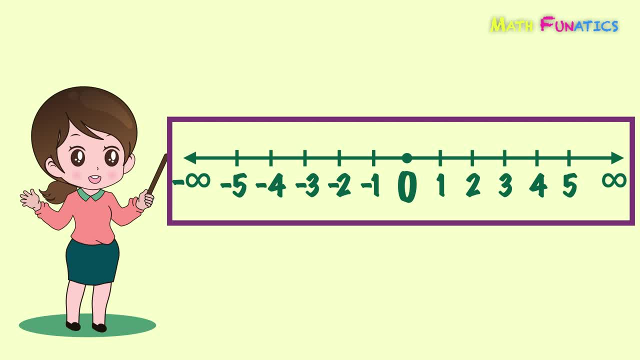 This entire set of numbers, from 1,, 2,, 3, and so on up to infinity, and negative 1,, negative 2,, negative 3, and so on up to infinity, and the number zero is what we call as integers. 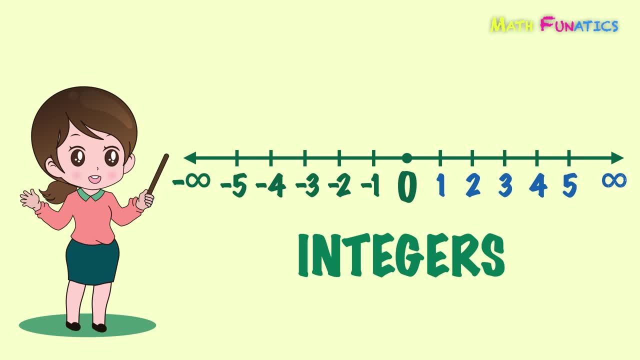 Integers that are greater than zero are called positive integers. They can be written with or without a positive sign. Integers that are less than zero are called negative integers. They must be written with a negative sign. On the other hand, zero is neither positive nor negative, meaning zero has no sign at all. 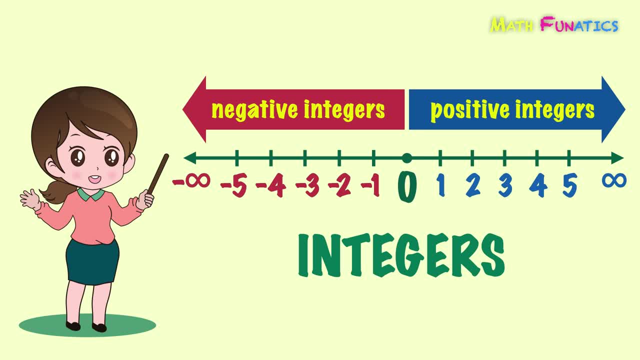 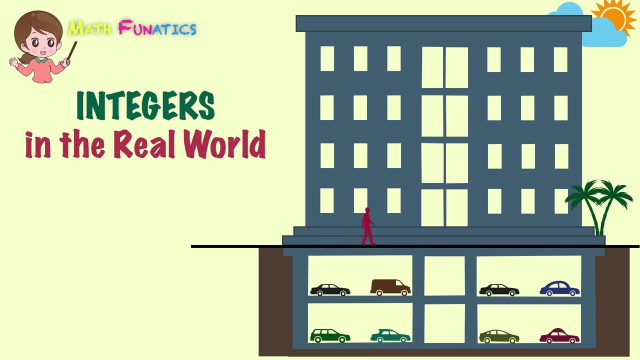 Furthermore, the set of positive and negative integers may also be called as signed numbers. To better understand integers, let us apply them in the real world. Let's take a look at this example: Going up and down a building may be related to integers. 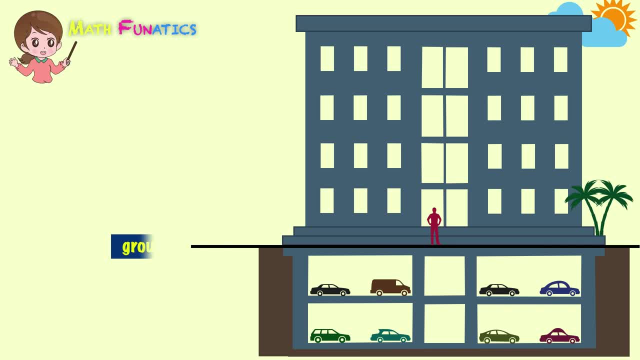 Let's see how it is done. The ground floor represents zero, while the upper floors represent the positive integers and the lower floors represent the negative integers. So if the man goes four floors up the building, then it may be represented by positive four or four. 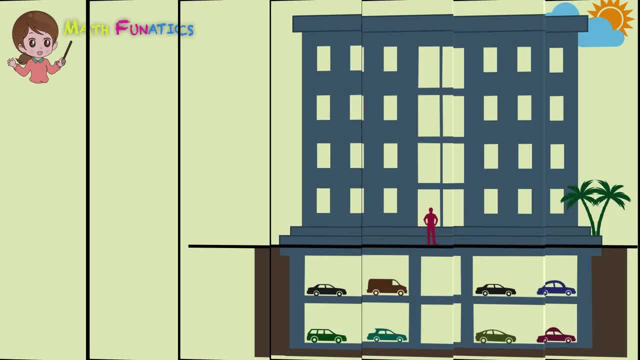 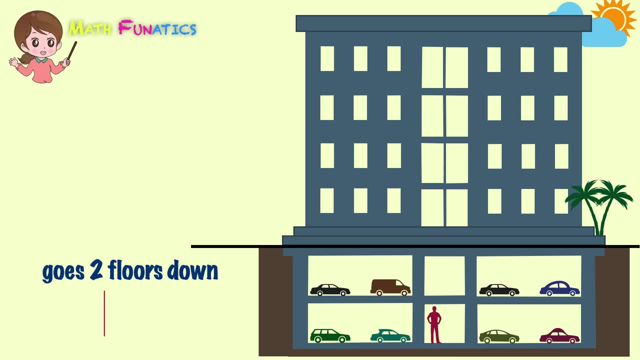 But if he goes two floors down the building, then it is negative two that best represents his action. To identify which integer best suits a given situation, we have to look for the keywords to give clues on what integers to apply. Looking back at our examples, the keywords that were used are the words up and down. 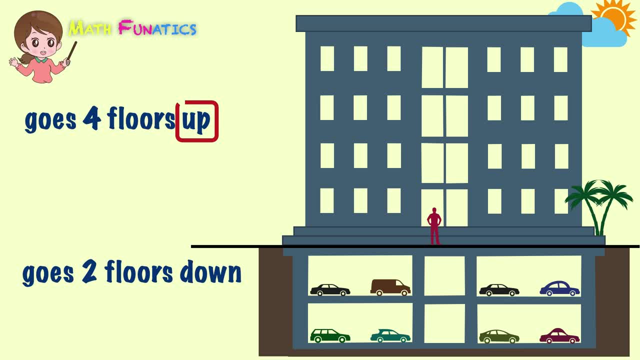 So when you encounter the word up or any other words related to it, it means that the integer is positive. That's why four floors up means positive four, And when you encounter the word down or any other words related to it, it means that the integer is negative. 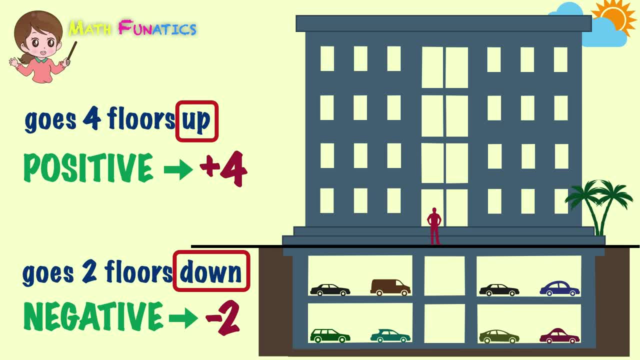 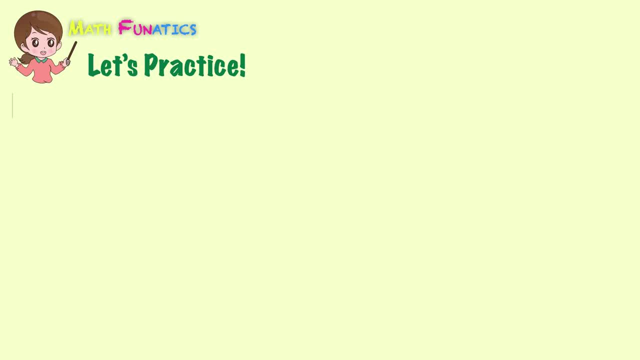 That's why two floors down means negative two. Now let's practice what the word up means, What you have learned about integers. Identify the integers that best represent the following situations: In the first situation, which is ten feet above the ground, 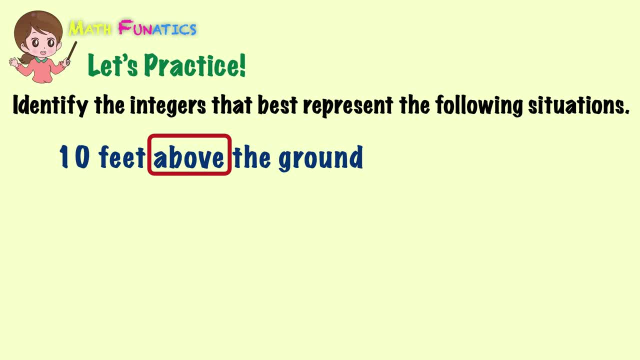 we see that the word that was used is above. Above means positive, So the integer is positive ten. Next, decrease of seven points. Next, decrease of seven points. Degree one from zero means negative, So the answer is negative seven.